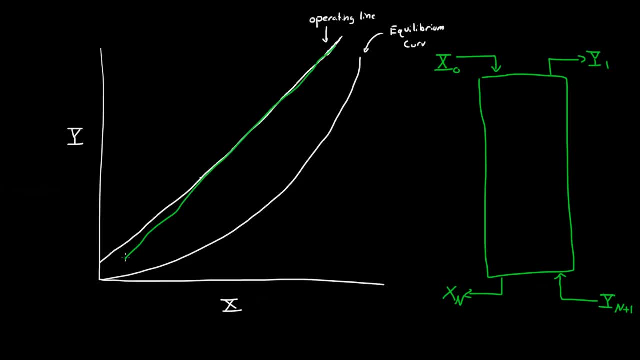 have the operating line. This is the operating line, It is always a line. And we also have the equilibrium curve, oops, curve, and it is set. we cannot change it. we can't have her change our operating line. and for instance, if we assume that 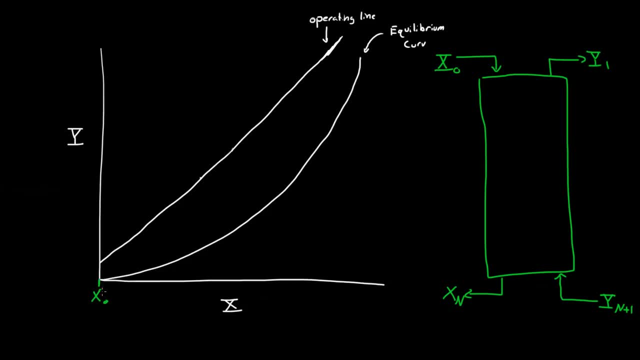 we have X naught. that is clean, so there is. so this is like high impurities in the liquid and this has no. this is like pure, clean liquid right here down here. so if we assume that we always had clean liquid and we wanted this to be y1, then 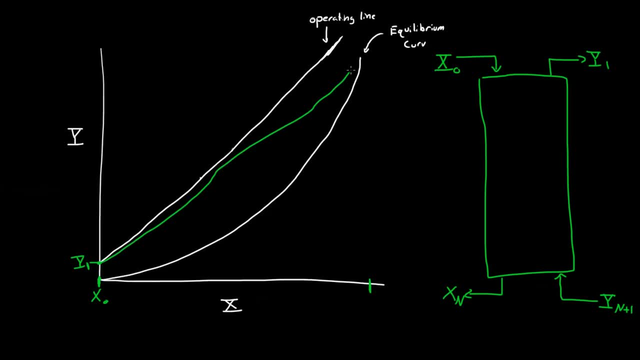 we could change how much the flow rates are and we get sorry, that's a bad drawing, but we could change the flow rates. we'd have it up something high like this or something like, something like this. but it's really important to note is that this operating line should never cross the equilibrium line and 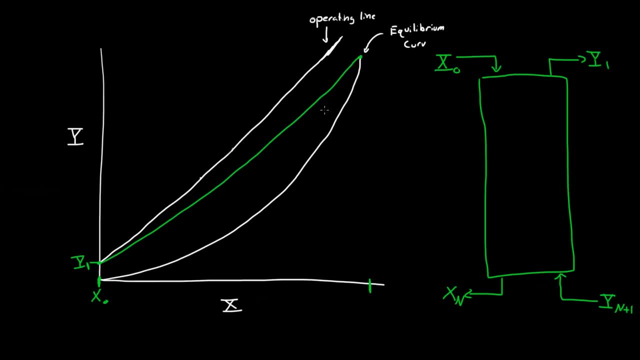 that will become hopefully clear in the next few minutes when I actually start showing you how the stages are made. so we know what y1 is and we and we know what X naught is. we assumed X naught was clean, so it'll be right here now. y1 is an equilibrium. 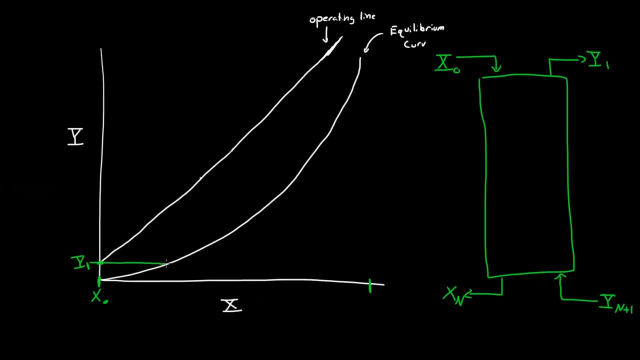 is an equilibrium with X X 1, so this is X- 1. so if we had stage 1, y 1 must be equal to 1. so if we had stage 1, y 1 must be equal to 1. so if we had stage 1, y 1 must be. 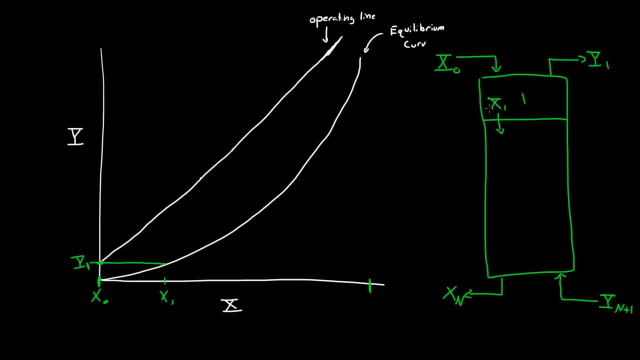 an equilibrium with X 1, X 1. so that is one stage, but X 1 is mixing with y2, it's mixing with y2, so we go straight up and this represents X 1 and y2, or their mixing point. you can kind of think of it. so this is y2. 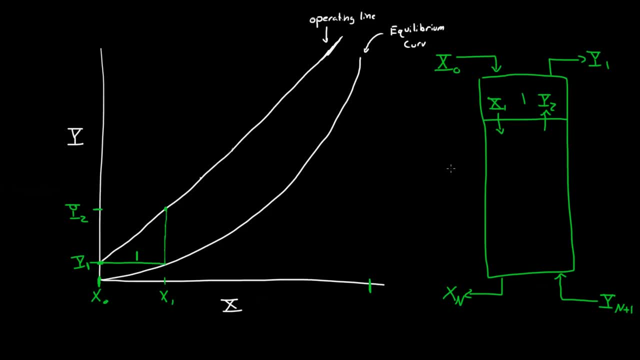 so that's their mixing point. but what? what is why? to an equilibrium with. so we have to go straight across to the equilibrium line from our operating line. an is an equilibrium with X 3, so we have another stage. this is stH two and it's an. 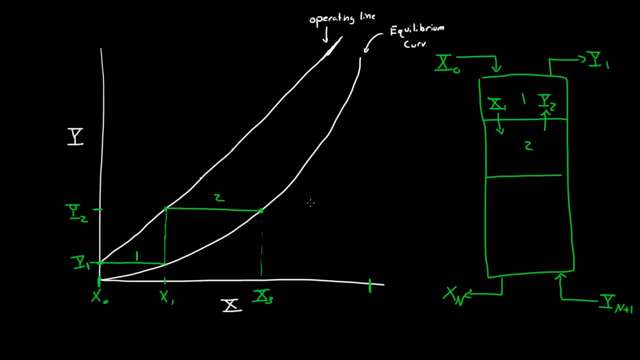 equilibrium with X 3. an x3 is mixing point 2. so what will I get next? so let's figure it out why, all of a sudden, I'm getting sth 1, but I need another X 1, so 3 is mixing with Y. Whoops, that's Y2, not 3, 2.. Oops, Because X2 is leaving stage 2,. 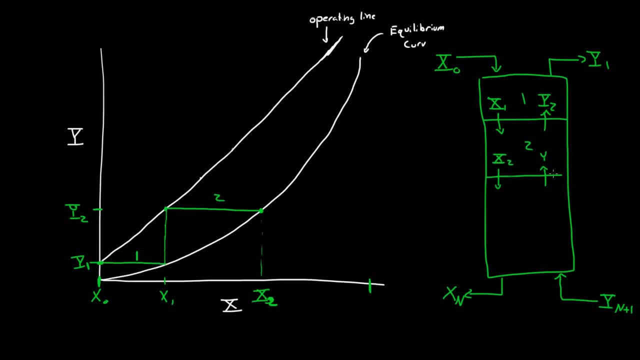 so these two must be in equilibrium with each other. And this is, of course, Y3, because it's coming from stage 3.. So we go up, and this is Y3. So we go all the way across. So what must Y3 be in equilibrium with? Well, Y3 must be in equilibrium with the liquid. 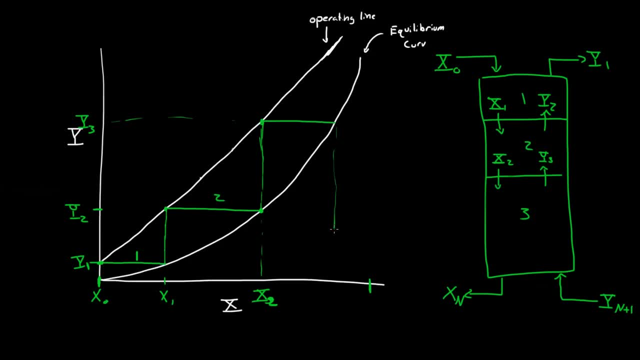 which is that which this would be X3.. So then, X3, oops, not doing that right. X3 must be is leaving, so it must be in equilibrium with Y3. And that is mixing with if we said that our, our containment, like this, was our should. 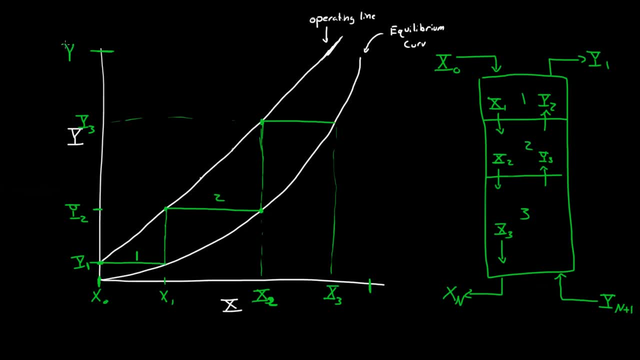 have done this at the beginning, but we knew our containment. our vapor had a containment of this amount or so. this would be N, So this was our containment. So our containment was mixing with the outlet. So then, if this is X3, then our contaminant, our, our vapor in the containment must be Y4. So we only 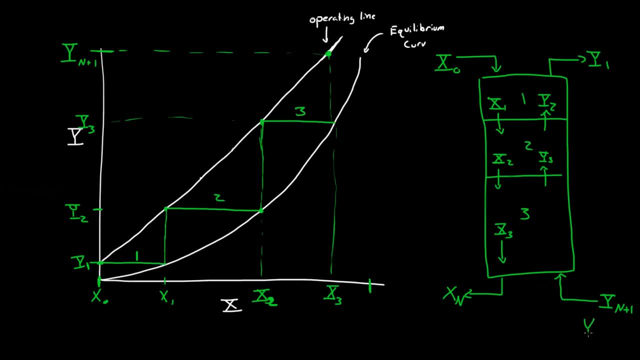 need three stages. So this is actually Y4, because X3 is mixing with Y4.. So this is Y4.. Okay, So really this is X3, and again just Y4. And again X3 is mixing with Y4, so mixing. 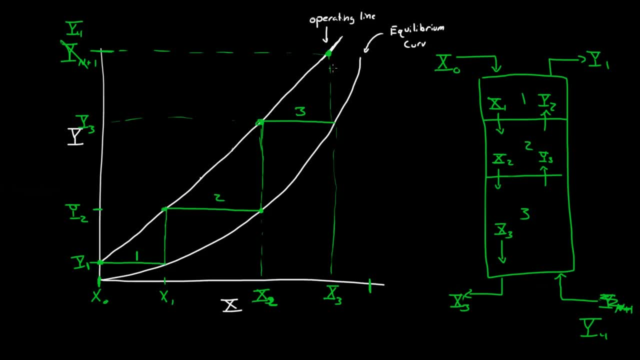 point, mixing point, mixing point. So it's really important that you have to start up here at Y, at Y4, or really you could just start right here. Maybe you're grappling something like this and if you know it's a straight line down, then you know that. 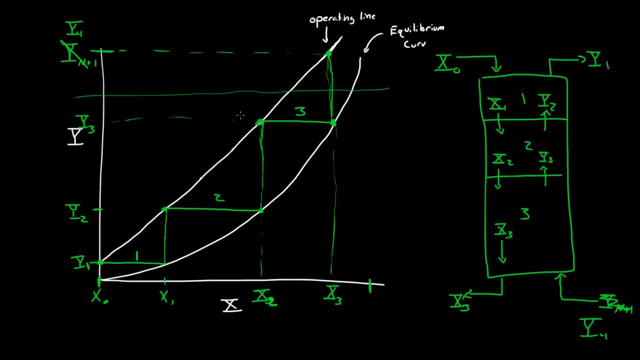 this is the equilibrium point and really the important thing is knowing that at this represents a state straight across, represents the number of stages. it's also important to know that that the the number of stages- this point has to hit perfectly- are this, this line that we go up and down and across each time, like 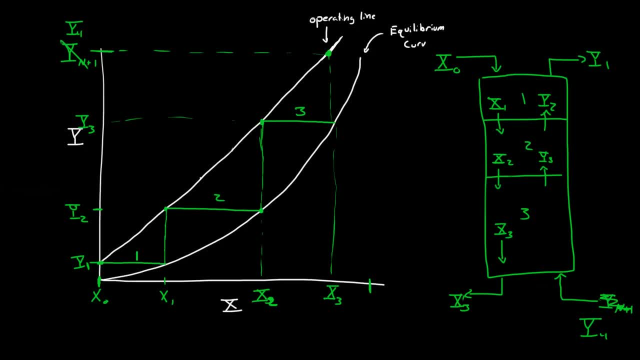 this must hit perfectly like that. so that's pretty much all there is to an absorption tower when you're trying to figure it out graphically. others actually a little bit more, and I'll go into it- about this operating line: how you can change this operating line. 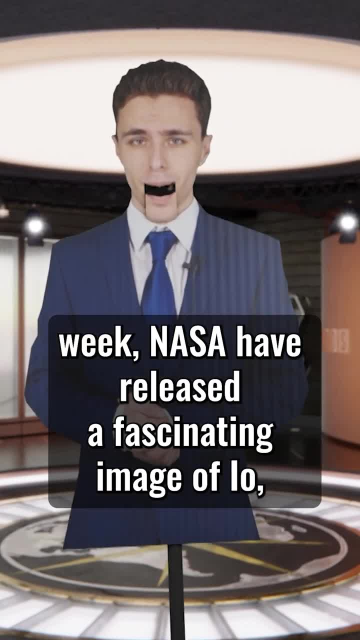 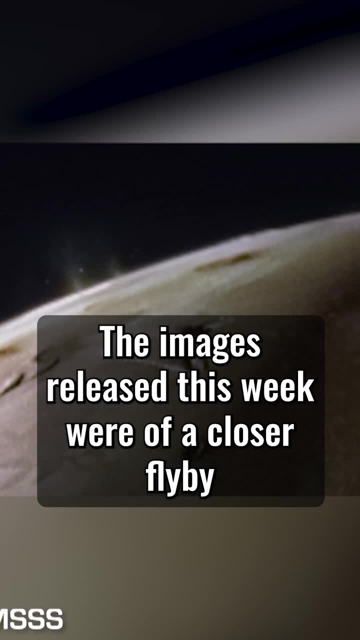 Starting off the news, this week NASA have released a fascinating image of Io, one of Jupiter's moons, after a close flyby on the 3rd of February. The images released this week were of a closer flyby and captured two active volcanic plumes. 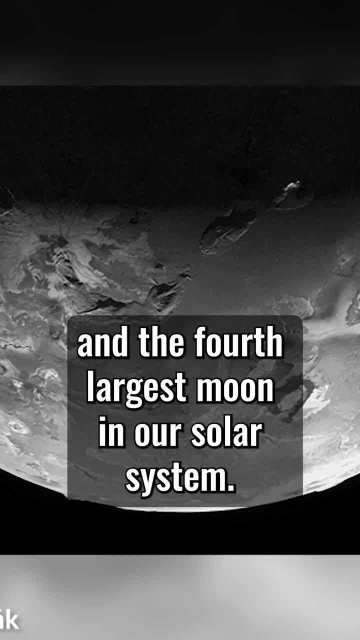 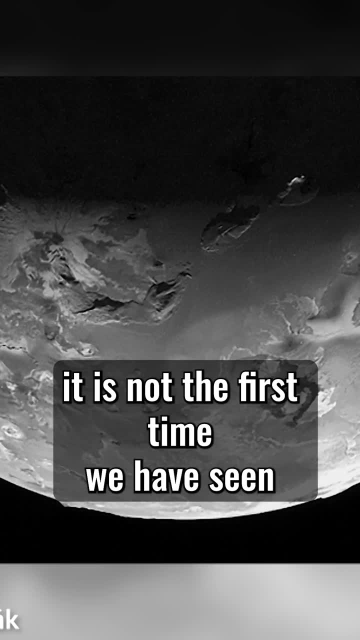 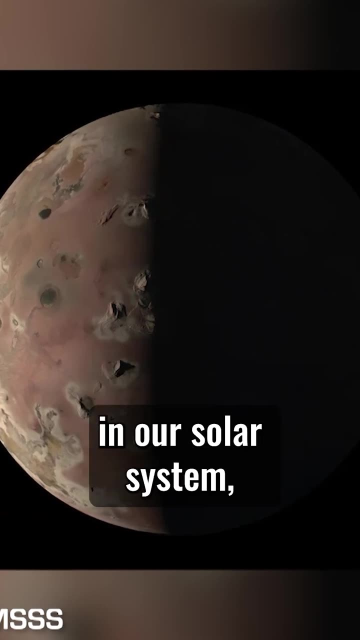 Io is the third largest of Jupiter's moons and the fourth largest moon in our solar system. While these images are both fascinating and crucial to our future understanding of the moon, it is not the first time we have seen its volcanic plumes. In fact, Io is the most volcanically active body in our solar system. 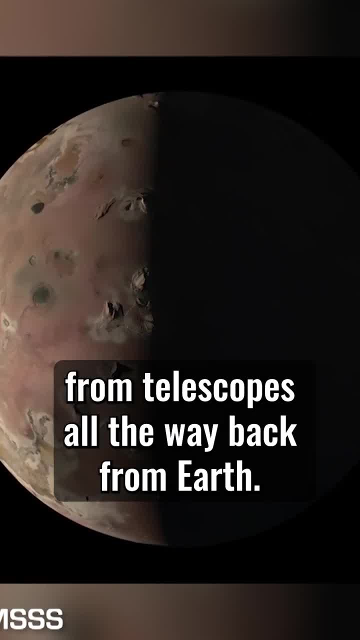 and its volcanic plumes can even be seen from telescopes all the way back from Earth.